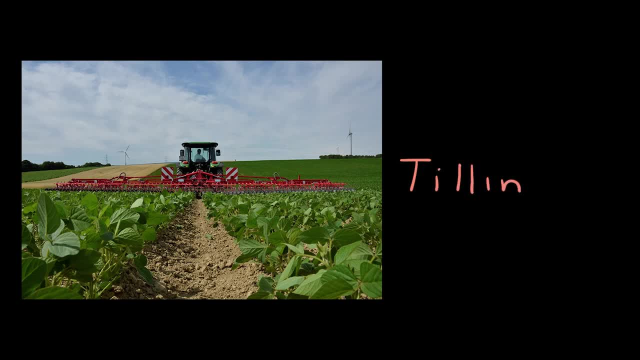 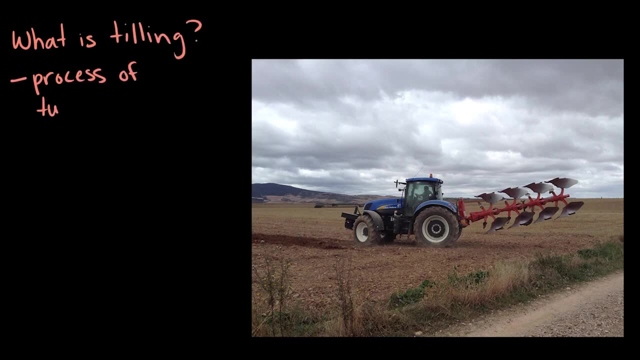 growing grains typically starts with tilling and good quality soil with lots of nutrients. But what is tilling? In short, tilling is the process of turning soil, And it's really useful because loosening the soil allows farmers to easily control weeds and other things. 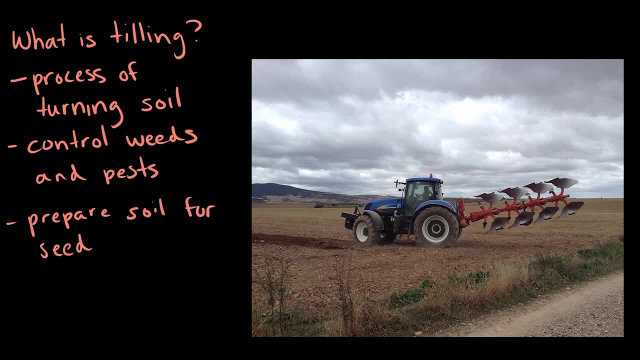 Soil is a good source of nutrients, And it helps them to prepare the soil for seeding. Sometimes, in areas that have been heavily farmed, the soil can become compacted over time. Here, tilling can help to break down the soil into smaller pieces. 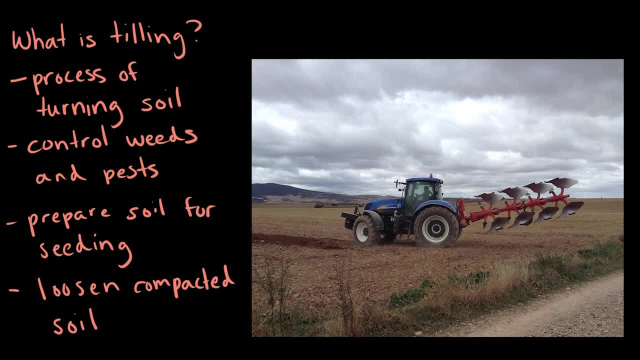 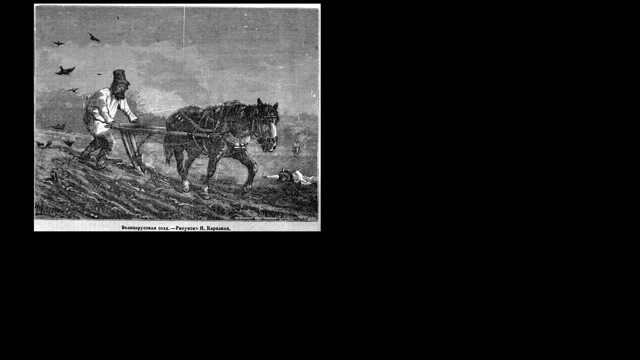 called soil aggregates and allow for easier crop planting. Now tillage has been done for thousands of years, But it's changed a lot from the past, when we used human labor and big draft animals to till small fields. But that's not all. 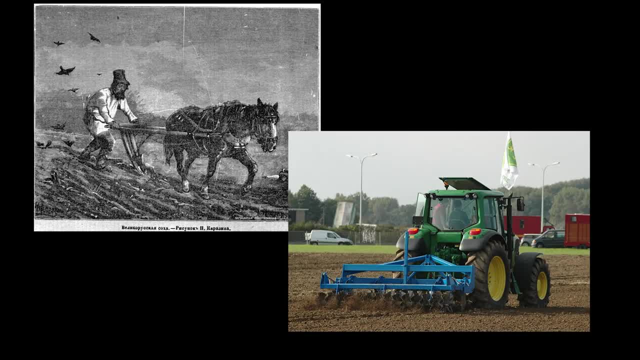 Usually once per year. Nowadays, in the era of industrialized agriculture, large scale farmers use heavy mechanized equipment that can till thousands of acres multiple times per year. OK, we're growing more, so we're tilling more, A lot more. 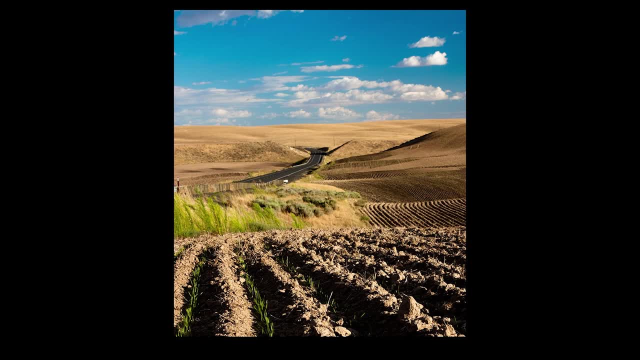 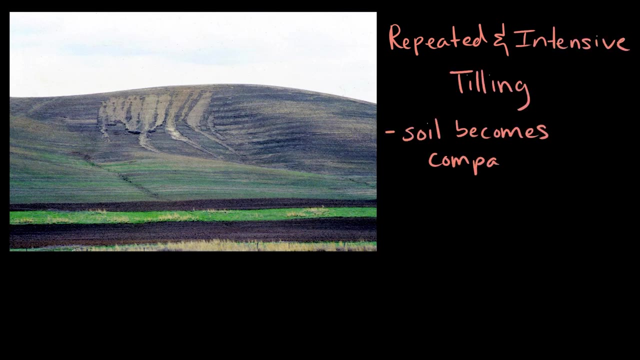 And while soil tillage can help to loosen and aerate soil, what do you think happens when heavy machinery passes over the land and tears up the surface multiple times per year? This practice of repeated intensive tilling compacts the lower layers of the soil and 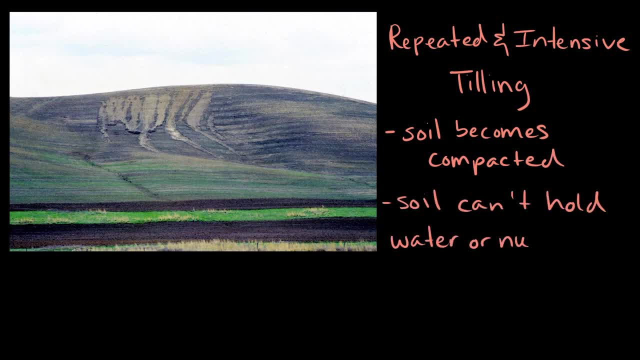 loosens the topsoil to the point that it loses the ability to hold water and nutrients in place. Tillage also reduces any leftover crop residue, like plant stocks. so in turn, the exposed soil surface becomes really vulnerable to wind and rain, because nothing is really holding the soil down. 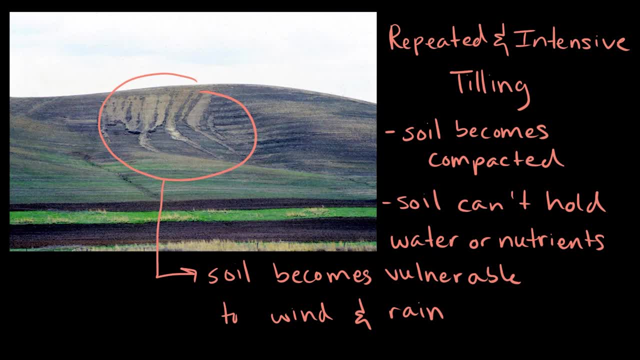 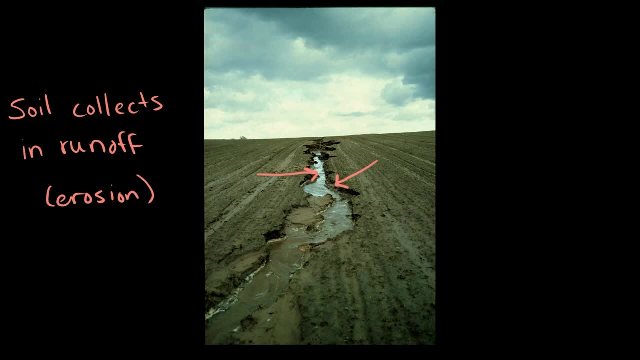 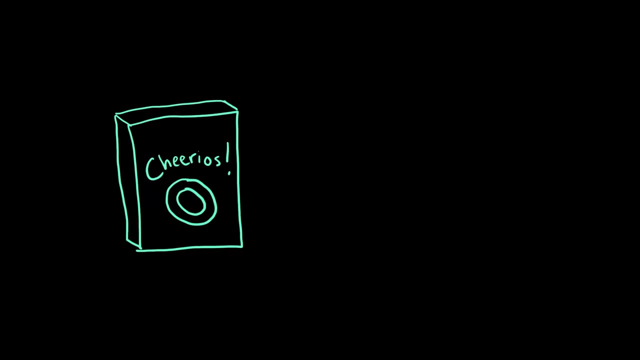 or providing cover. So what happens next? Loose soil can start to collect in surface runoff and become displaced through erosion. When this happens, soil, organic matter and nutrients are literally washed or blown away. Who would have thought that these Cheerios were doing so much? 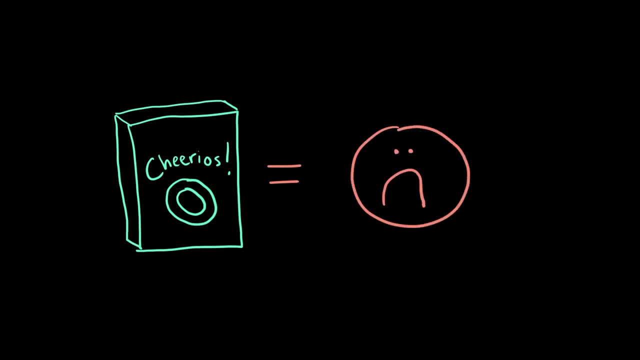 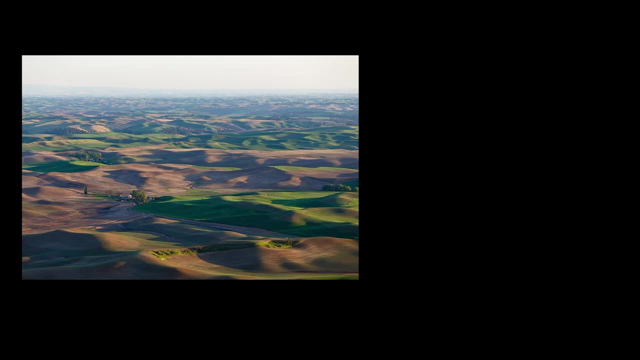 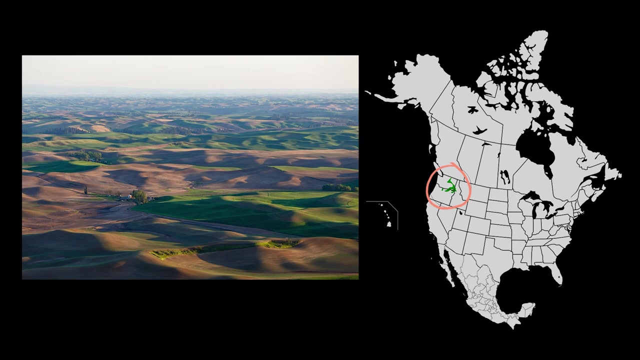 damage. But there's some good news here too. Low-till or no-till farming alternatives can alleviate some of these problems. thankfully, In the Palouse, a huge agricultural area in the western US where a lot of grains just like the ones in my cereal are grown, no-till farming is really important because the 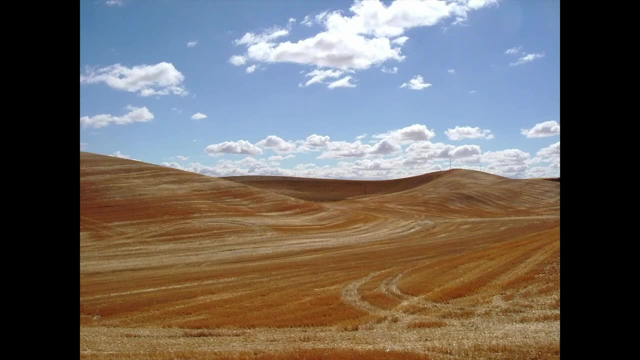 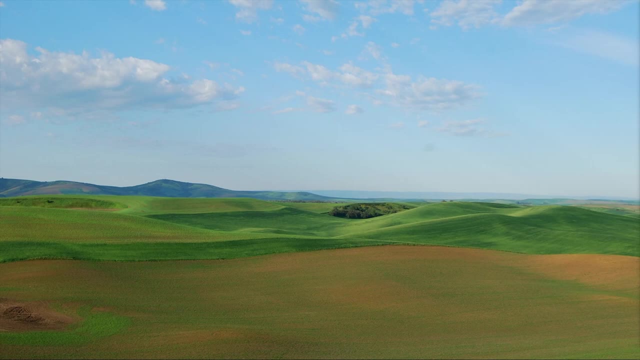 fields are well. they're really steep and hilly and wind and rain can cause a lot of erosion when the soil is heavily tilled. By not tilling the fields, farmers can prevent soil erosion and, more importantly from my perspective, make sure that they can grow lots of grains for my Cheerios. 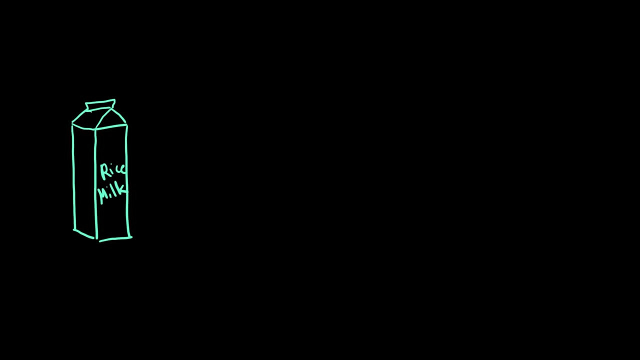 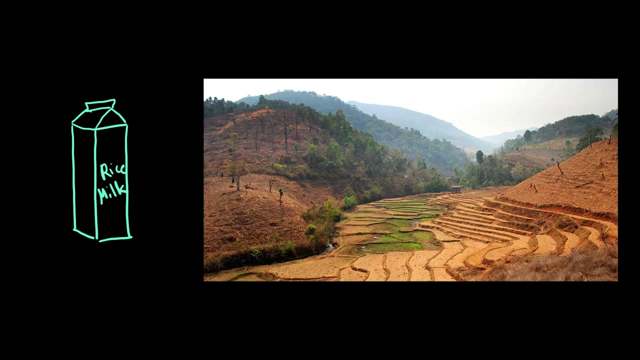 But wait, cereal isn't complete without milk. Now, I personally like rice milk because I'm lactose sensitive, and rice is commonly grown in temperate and tropical regions, oftentimes in areas where soil quality isn't the best and nutrients are lacking. 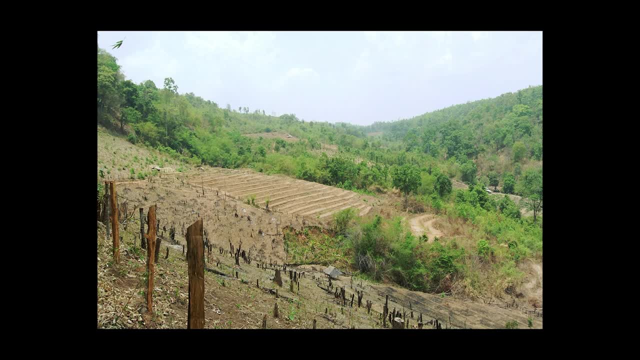 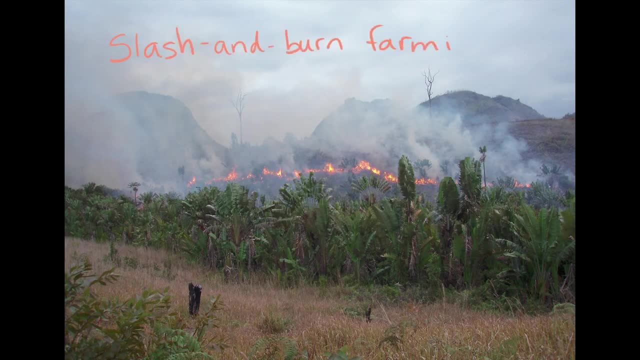 So how do farmers get nutrients back into the soil And, more importantly, how do they grow rice for my rice milk at breakfast? Well, they often use slash and burn farming. So, like the name, forest plots are slashed or cut, left to dry and then burned. 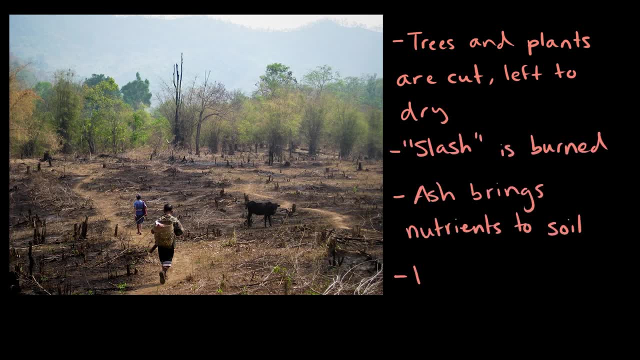 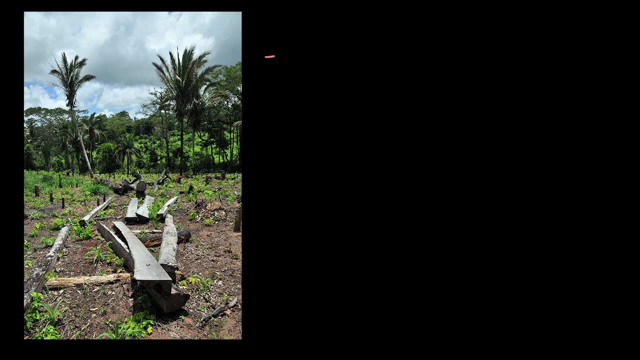 The ash left over from the burning fertilizes the soil, but it's only a temporary benefit. After about three to five years, the productivity of slashed and burned plots goes down really quickly due to the loss of nutrients and as weeds start to grow again. 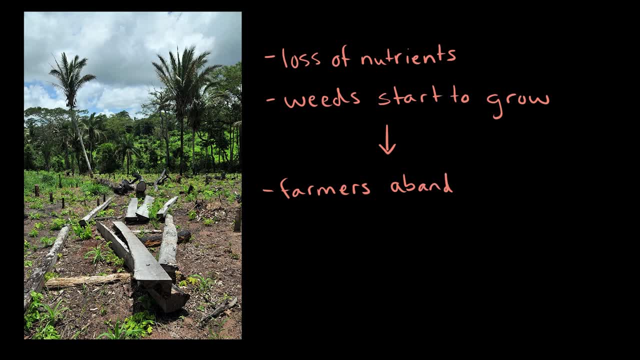 When this happens, farmers simply abandon the field, move over to a new area and repeat the process, But it can take decades for these plots to recover once they've been slashed, burned and farmed, and this practice can become a vicious cycle. 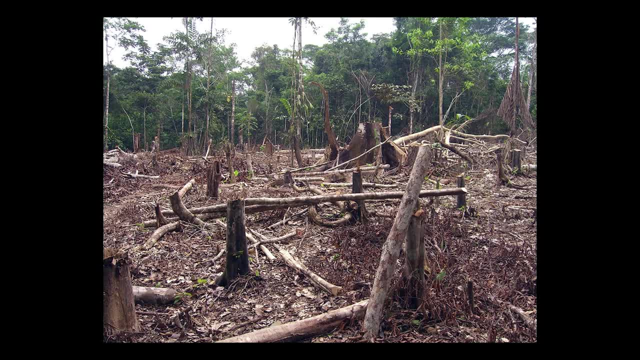 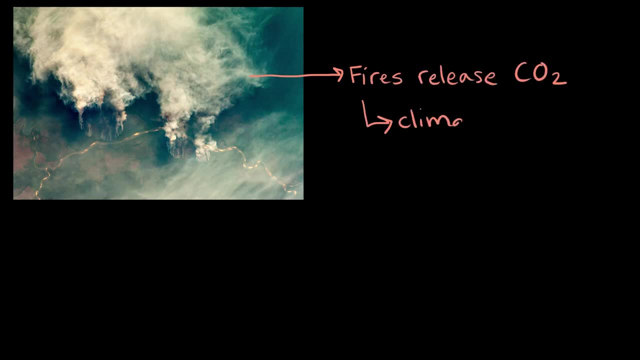 In the Amazon, for example, people in rural areas rely on slashed and burned so that they can make money selling the crops they grow or create open pastures for animals to graze. In the process, thousands of acres are burned each year, And as these trees and plants burn, enormous amounts of greenhouse gases, mainly carbon dioxide, are produced. 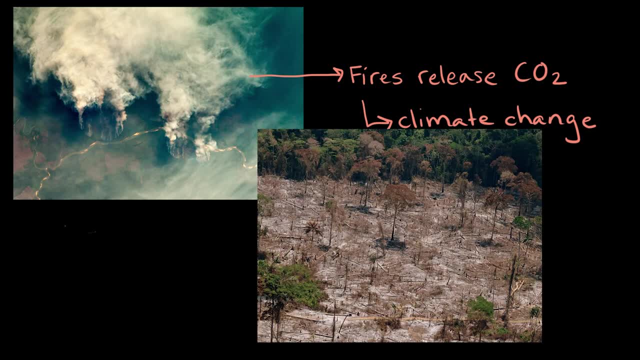 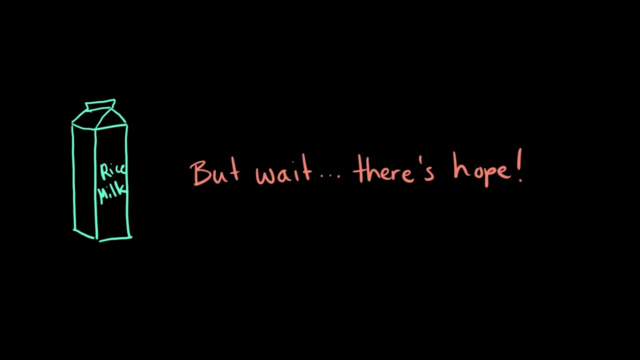 Which contribute to climate change. And sometimes too, fires may not be well managed and can burn out of control, causing huge, costly wildfires. But it's not all doom and gloom when it comes to my tasty rice milk. There are alternatives to slashed and burned, which include applying animal fertilizer like manure on used plots to bring nutrients back to the soil. 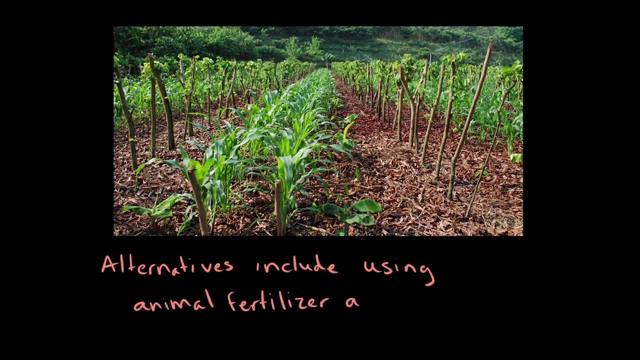 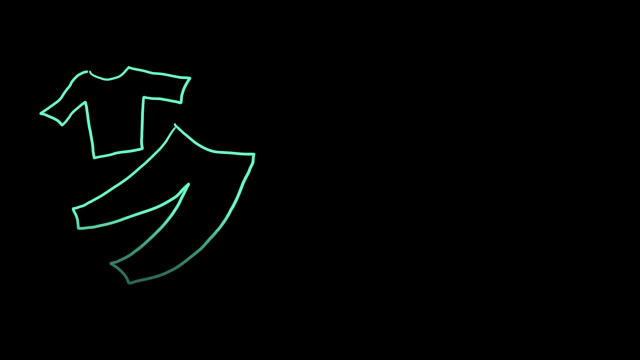 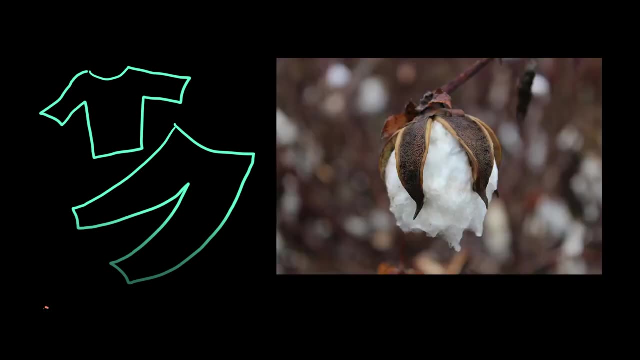 Or using alley cropping, in which trees or other vegetation are planted between crops, to help keep nutrients and moisture in the soil. Alright, by now I've eaten my breakfast and I'm relaxing in my super comfy cotton pajamas, But turns out that cotton is actually a really finicky crop to grow and it requires a lot of fertilizers. 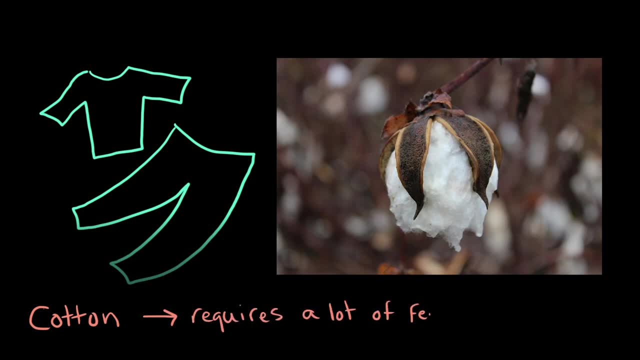 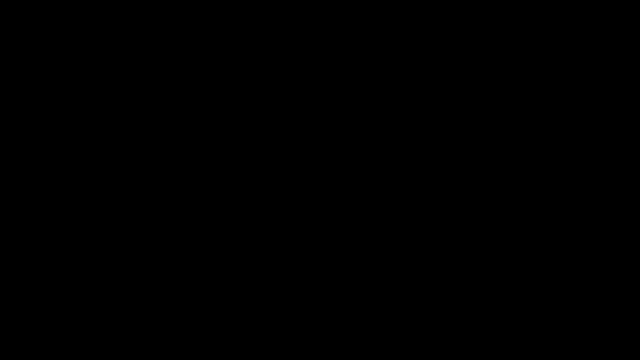 And fertilizers help plants growbut that's not a bad thing, right? And it's not. In fact, we've been using fertilizers for millennia. For thousands of years, people have used natural fertilizers to replenish or increase nutrients in the soil. 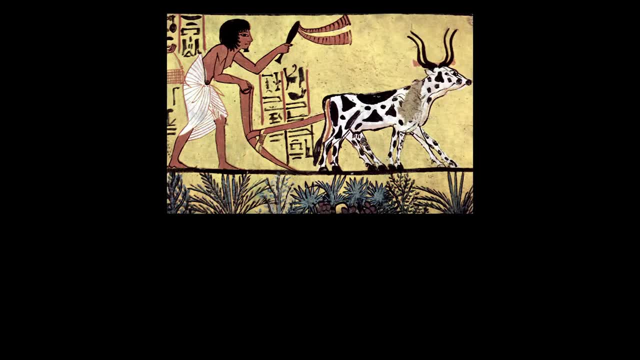 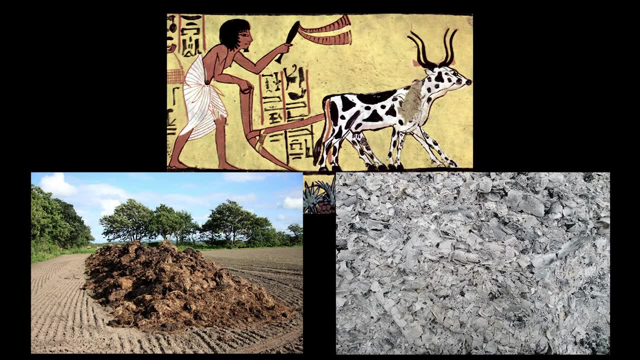 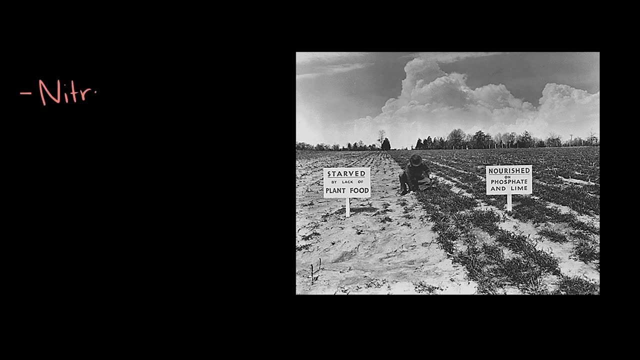 And that's not true, No, it's not- and promote plant growth. Natural fertilizers meant that farmers used things like leftover crops, manure, wood ash, ground bones, fish or fish parts, and even bird and bat poop. In the early 1800s, though, scientists discovered that nitrogen, phosphorus and potassium were key. 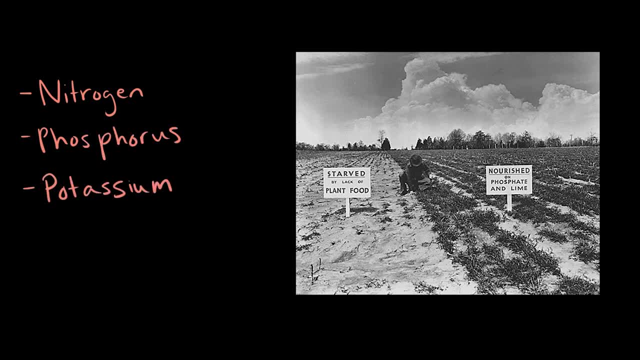 to plant growth And in time, many farmers began to switch from natural fertilizers to artificial fertilizers with higher concentrations of these nutrients, which greatly increased crop yields. In other words, farmers could grow more, and that means more cotton and more comfy pajamas. 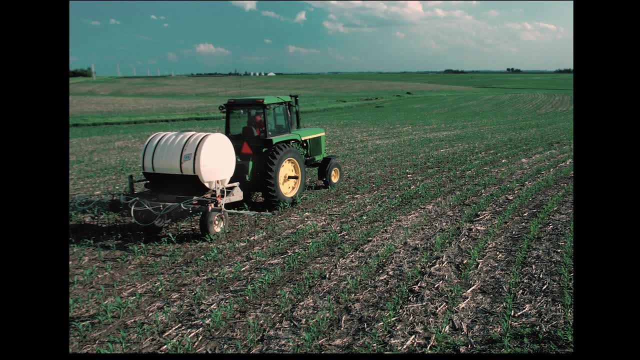 But there's a catch. Now that farmers are growing more crops than any time in history, we've learned that there are impacts to using large amounts of very concentrated fertilizers. Applying too much fertilizer can pollute runoff water with excess fertilizer and pollute local. 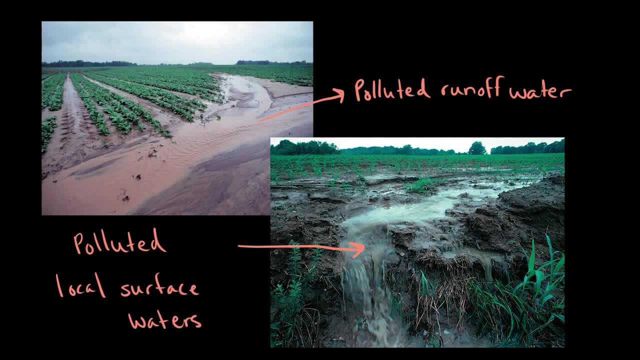 surface waters. As nutrient-rich materials like fertilizer make their way into nearby rivers, lakes and oceans, they can cause major problems in the balance of nutrients in marine ecosystems When too many nutrients from fertilizers saturate a body of water called eutrophication. 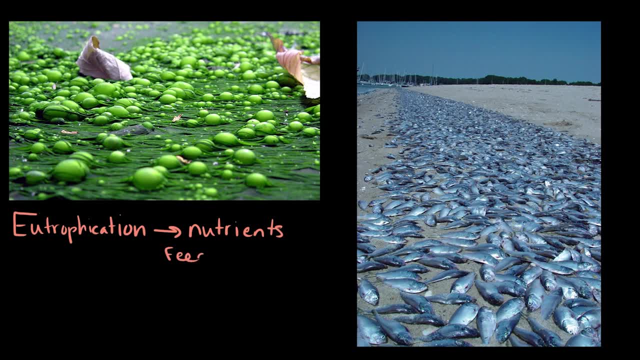 these nutrients feed the rapid growth of algae. In turn, these massive algae blooms can suck up all the oxygen in bodies of water and lead to enormous fish die-offs, called dead zones. Quite a morbid situation, and very different from the happy unicorns in my pajamas. 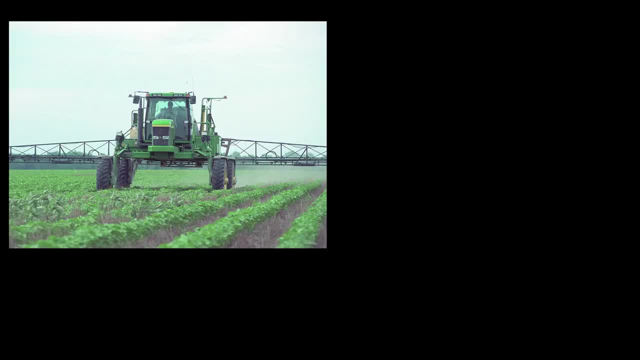 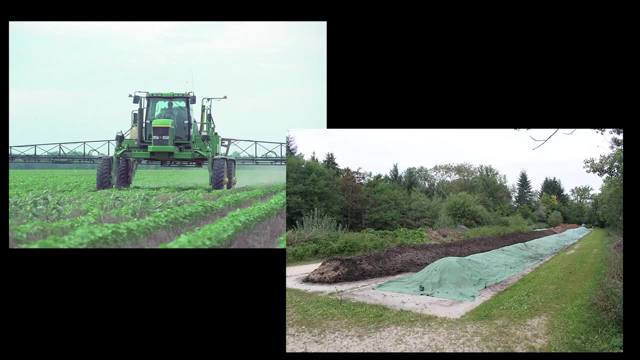 But there's ways to reduce this. Farmers can limit the amount of fertilizers released into waterways. Farmers can limit the amount of fertilizer that they apply or use compost, which is decomposed organic material, as a fertilizer, which tends to have lower and safer levels of nitrates and phosphates. 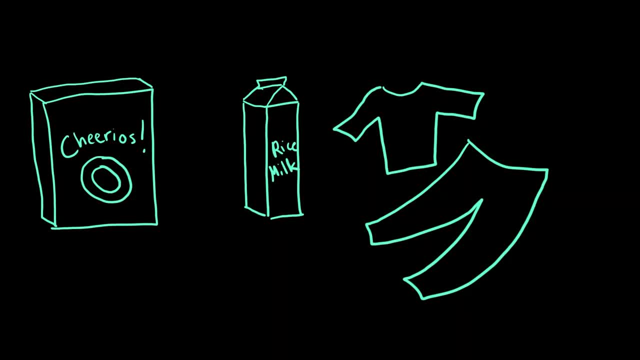 And there you have it: Common agricultural practices and their impacts in a nutshell.